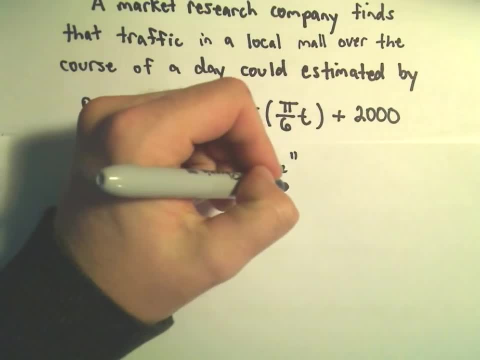 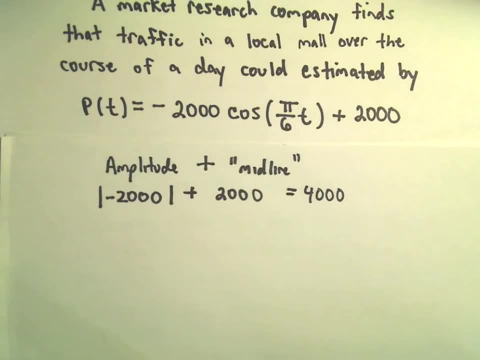 Well, the absolute value of negative 2,000 plus 2,000 is going to be 4,000.. So I think that's going to be the maximum number of people, But let's talk about trying to get that value, maybe by graphing. 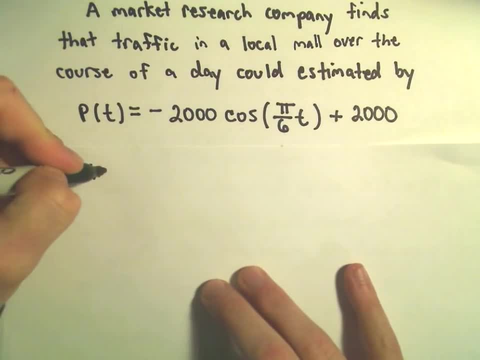 Okay, so a couple of things. The amplitude we just said was going to be positive 2,000.. Again, we have to take the absolute value, The period. so let's think about the period. Again, the period is 2 pi over the absolute value of b. 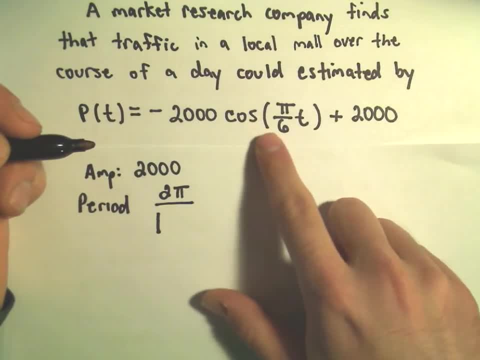 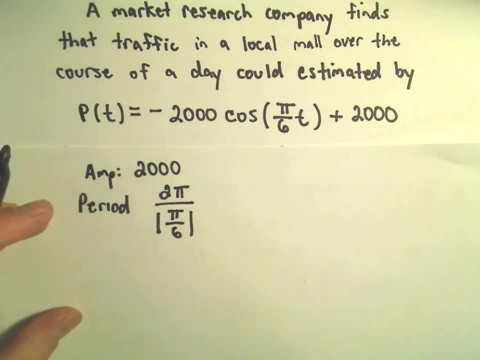 b is whatever number is in front of the variable, you know, sort of inside the cosine or sine function, which is going to be pi over 6.. Okay, the absolute value of pi over 6 is just pi over 6.. So I'm going to think about 2 pi as being, well, 2 pi over 1.. 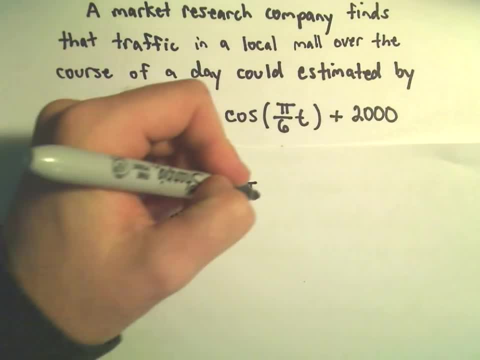 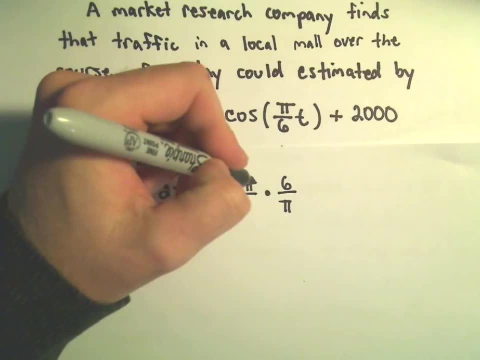 If we have pi over 6 in the denominator, if we're dividing by that, that's equivalent to multiplying by 6 over pi. So in this case the pi's would cancel 2 times. 6 is going to give us 12.. 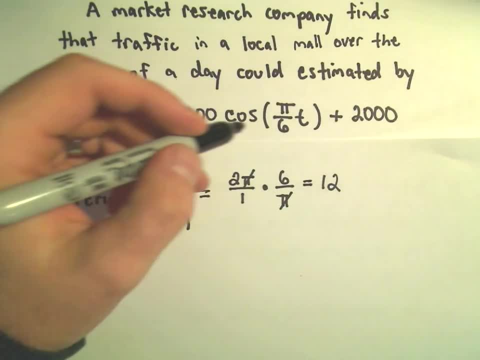 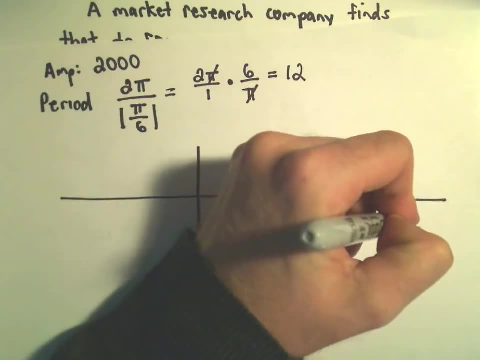 So it says our cosine function here, our cosine graph, is going to have a period of 12.. All right, so let's see, I'm going to go all the way out here to 12. And I usually break it up into, you know, kind of four pieces, so four little equal sections. 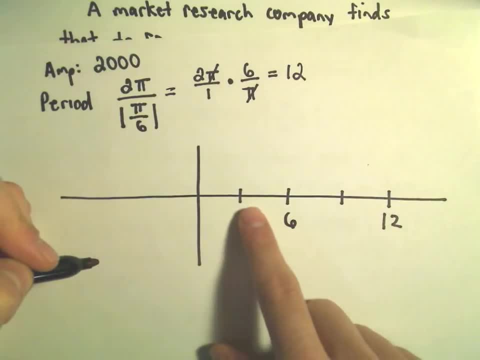 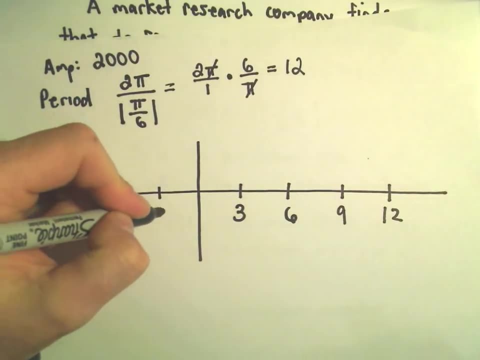 So if the period's 12,, half of that is 6.. Half of 6 would be 3.. So all my increments are going to be in 3s, which would make this 9.. Likewise, negative 3,, negative 6,, et cetera. 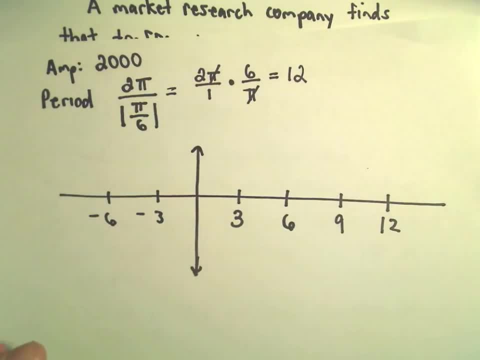 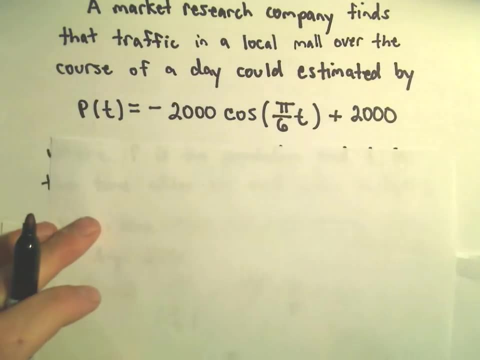 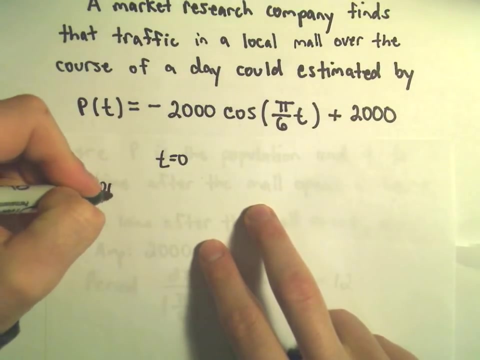 So let's just try to, you know, maybe plot some points and just graph this function and get a feel for what's going on. So let's see, Maybe we can plug in. let's plug in: t equals 0. If we plug in t equals 0, it says the population. 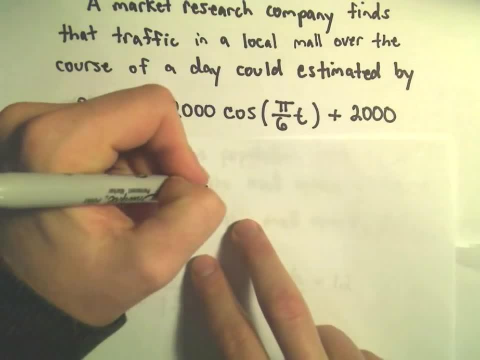 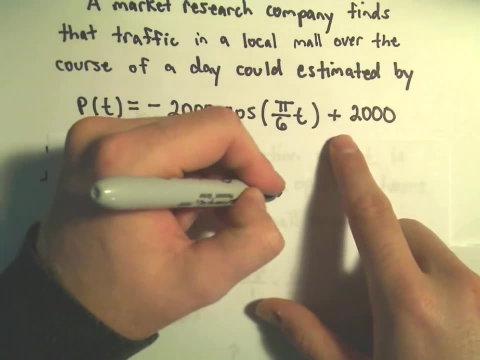 at time 0 would be negative 2,000 times cosine. Well, if we take pi over 2, that would be negative 2,000 times cosine. So if we plug in pi over 6 times 0, we'll just get 0 plus 2,000. 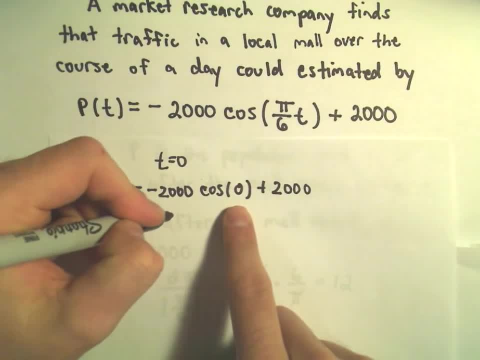 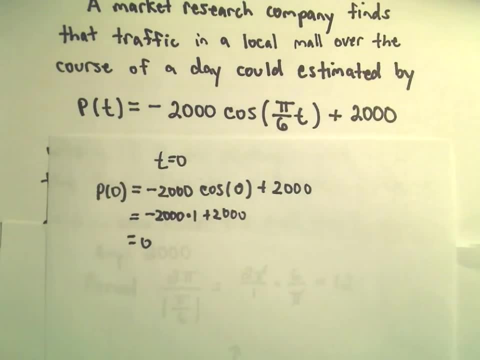 Cosine of 0 is 1.. So we'll really get negative 2,000 times 1 plus 2,000.. Or we'll actually get 0 out. So all this says is: at time 0,, the population is 0.. 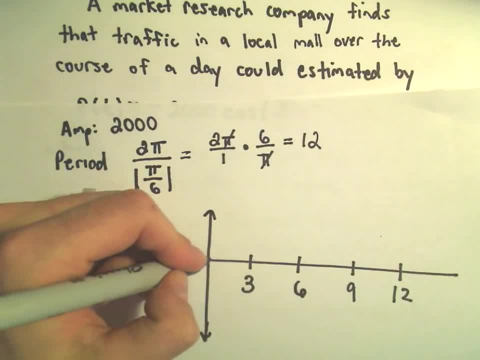 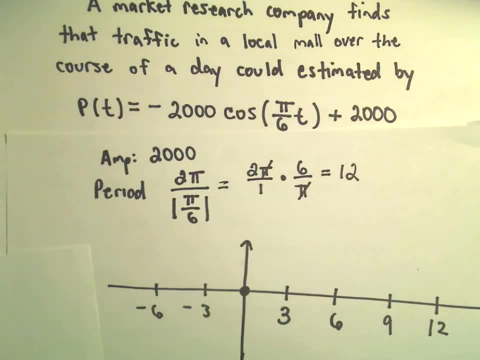 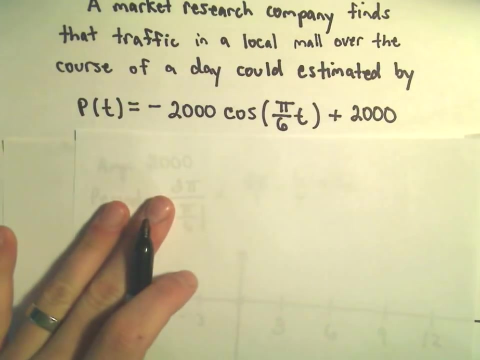 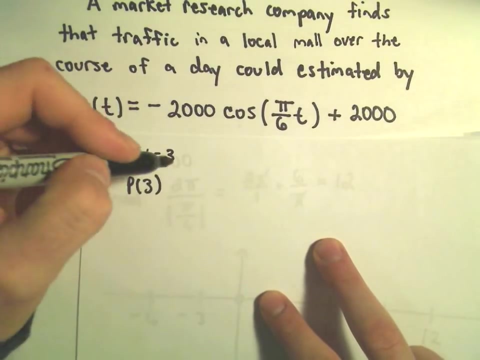 So maybe they're closed at that point. All right, let's plug in a few more points here as well. Maybe let's plug in 3 and 6 as well, to see if we can't figure out what's going on. So if we plug in, t equals 3, we'll get the population after 3 hours is negative 2,000 times cosine. 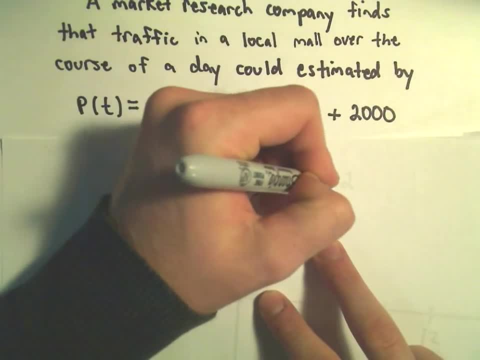 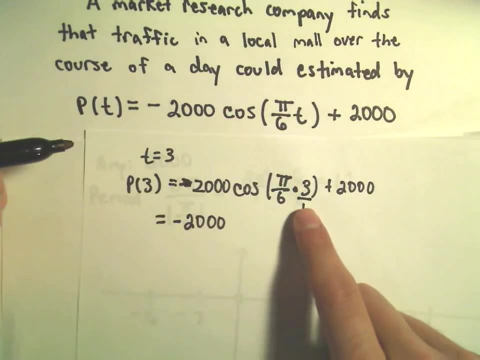 We'll have pi over 6 times 3 plus 2,000.. All right, You can think about 3 as just being 3 over 1.. So we have 3 over 6, which is going to give us pi over 2.. 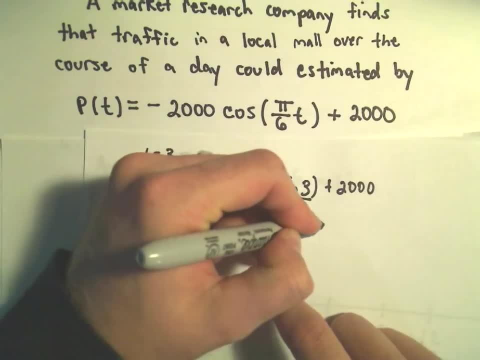 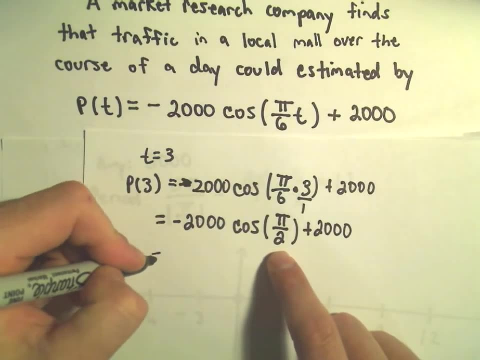 So we have cosine of pi over 2 plus 2,000.. But cosine of pi over 2, that's just simply equal to 0. So it looks like to me the population after 3 hours is just going to be 2,000. 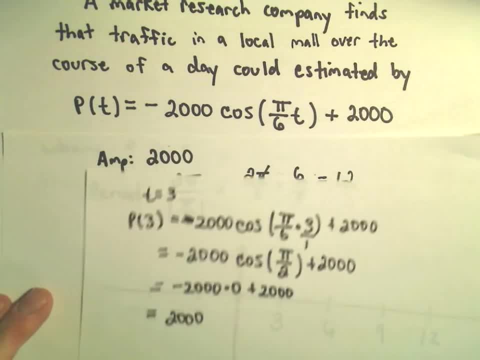 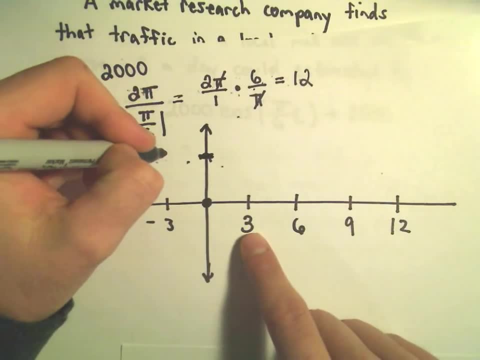 2,000, 2,000 people. Okay, so let's go back. So I think we said: at zero there's zero. I should have made my graph a little bigger. Let's see. after three hours We said there's 2,000 people. 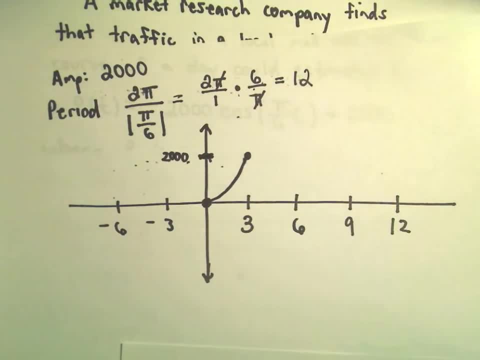 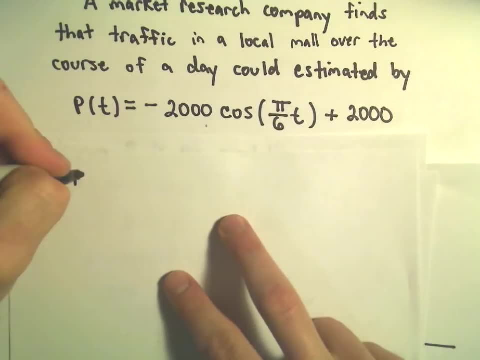 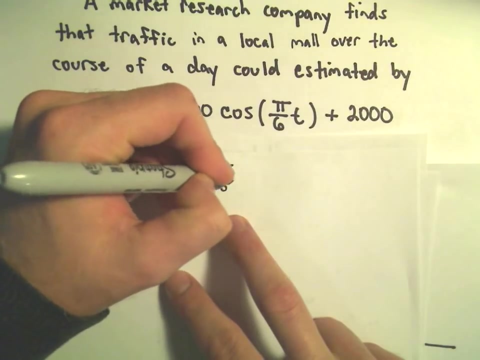 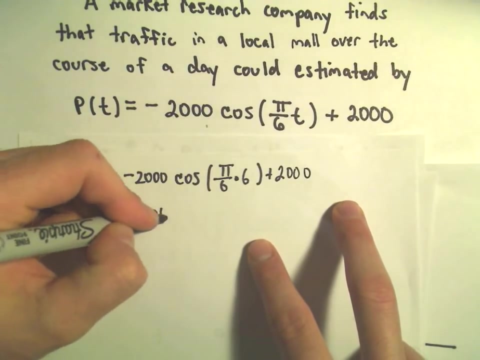 Maybe let's plug in just one more value here. Let's plug in: t equals 6, so the population at times 6, we'll get negative 2,000. We'll get cosine of Pi over 6 times 6 plus 2,000. Let's see this would give us 6 Pi over 6 or just cosine of Pi. 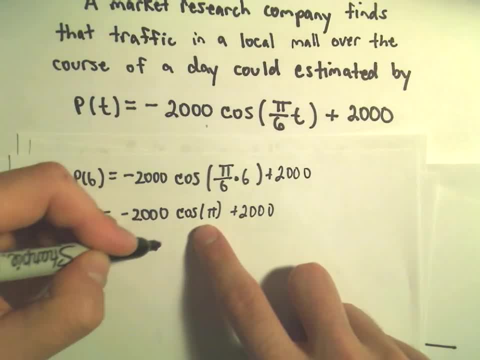 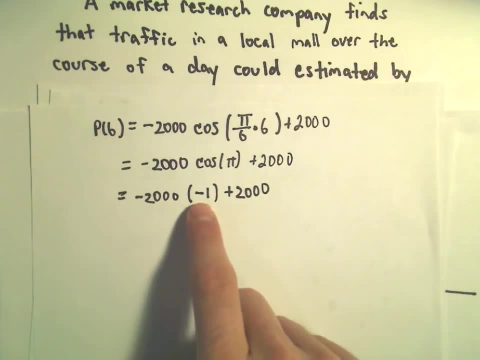 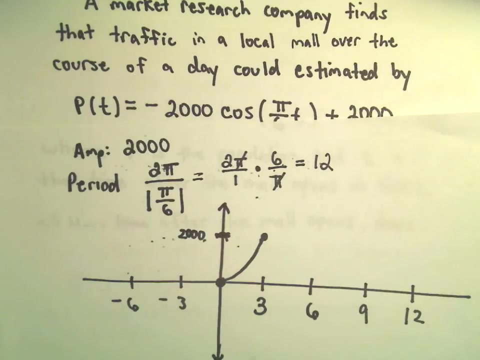 plus 2,000. Well, cosine of Pi is negative 1, So really we're getting negative 2,000 times negative 1, which is 2,000 plus 2,000.. We're actually getting our population now to be 4,000. 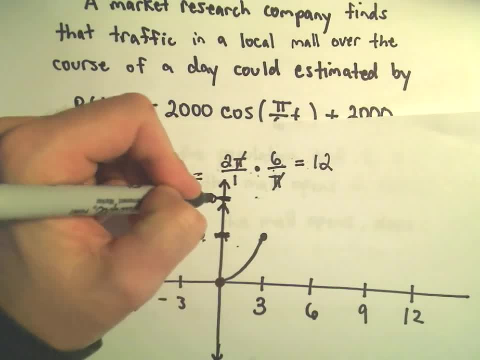 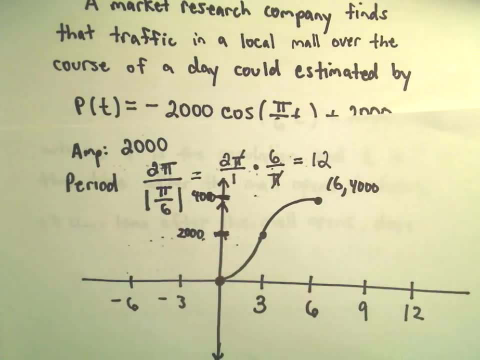 So okay, at t equals 6.. We're actually up here at the population of 4,000, And now you can always plot some More points. you can plug in 9. what's going to happen is you're going to be back down here at. 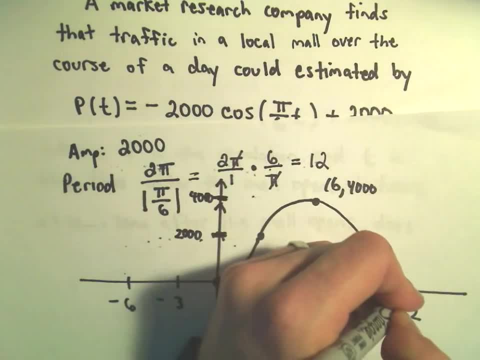 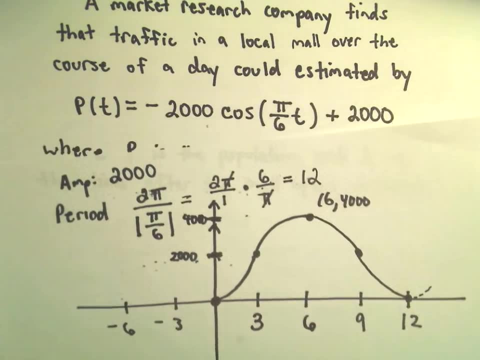 2,000, and then when you plug in 12, you're going to be back at 0, and then again We said that's, the period is 12, so it's now just going to start repeating itself. So it's kind of a cosine function. 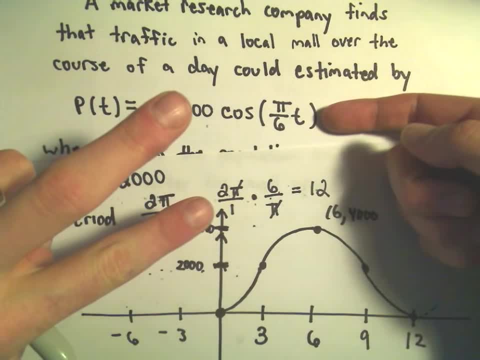 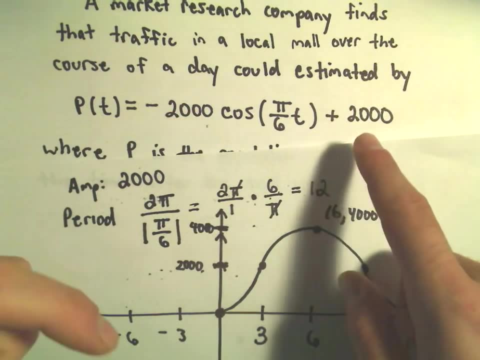 That's been flipped about the x-axis. You know the original cosine function. the Pi over 6 has stretched out the period, the negative 2,000 has flipped it about the x-axis and then the positive 2,000 has shifted that graph up some up 2,000 units. so 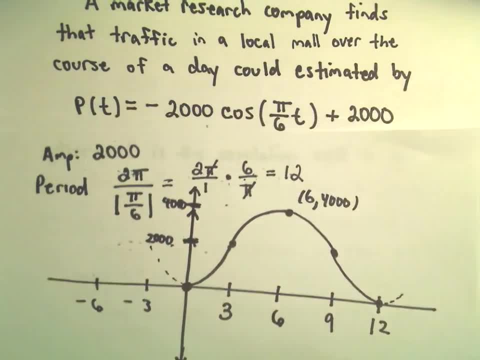 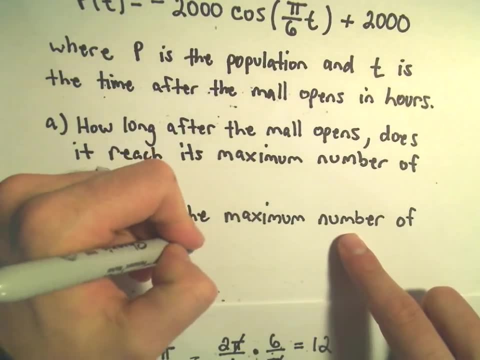 But now, with this decent graph, I think we can answer all of our questions. so we said: How long, let's see. so I think we already answered part B. What's the maximum number of people- we made an argument about that at the very beginning- which is just 4,000?. 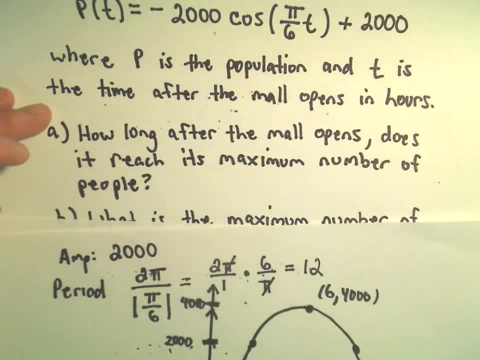 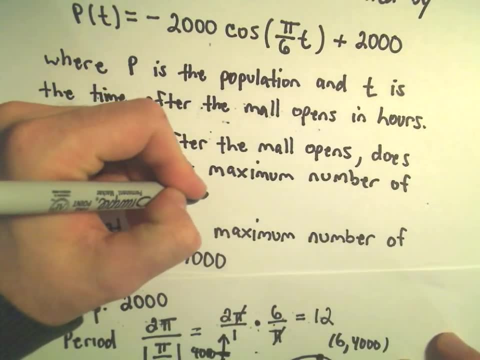 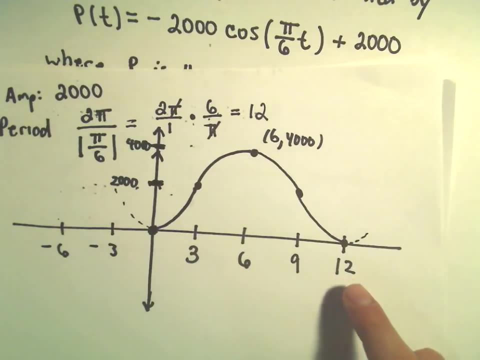 Well, it says how long after the mall opens does it reach its maximum number of people. well, the first time it reaches its maximum number of people would be six hours later, and Then after 12 hours it would be empty, and then it looks like if you add another six hours to that, we would be 18 hours. 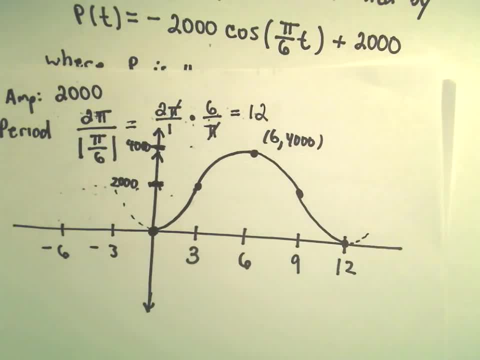 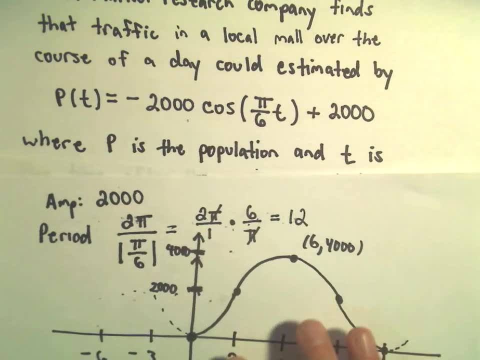 So that would be kind of the second time It's at its peak capacity. so again, You don't have to do this necessarily by graphing the function. you can always sort of give an algebraic argument. But you know, again, it never hurts to to think about the graph. to me if I have a nice good graph,